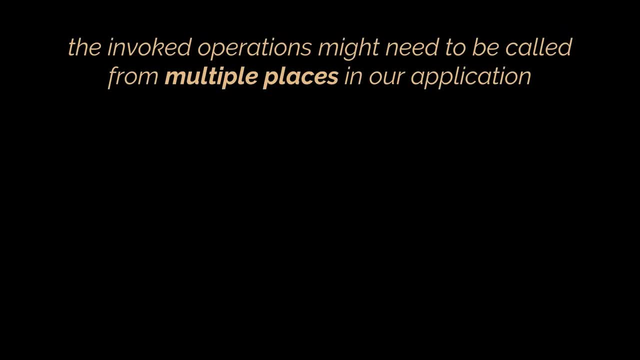 part. The operations you are invoking might need to be called from multiple places, like not just from the house rooms we created. What I mean by that is that the operations you are invoking- is suppose the application we are developing- can now switch any light in the house, not just room. 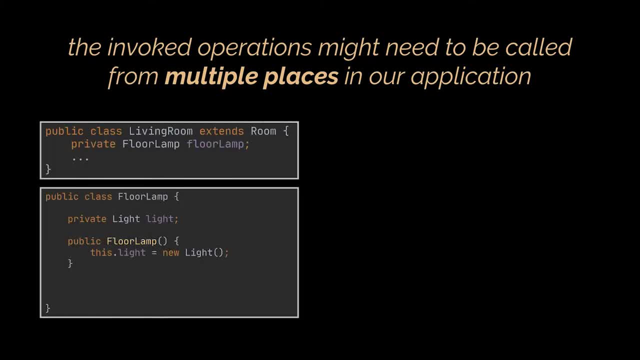 lights. So if we add a floor lamp in the living room and want to use our application to turn it on and off, we can't let the floor lamp class extend the room class because, simply, it's not a room. Therefore we will have to duplicate the lights- logic we wrote for rooms inside the floor. 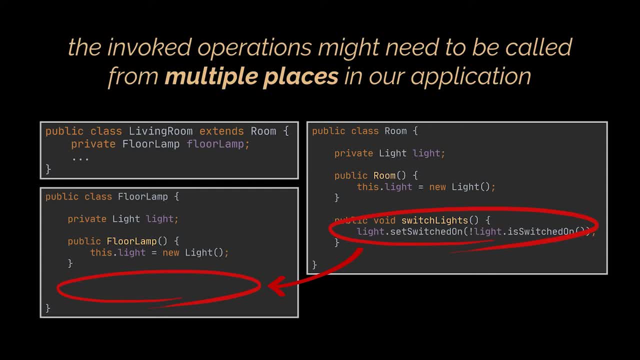 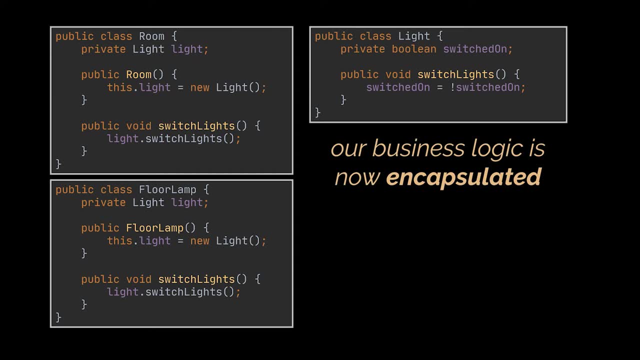 lamp class. To avoid this, what we can do is first move the light switching logic from the room and floor lamp classes to the light class itself. Doing this, we encapsulated the light switching logic inside the light class so that any time we change this logic, it will be modified across all the parts of our application. 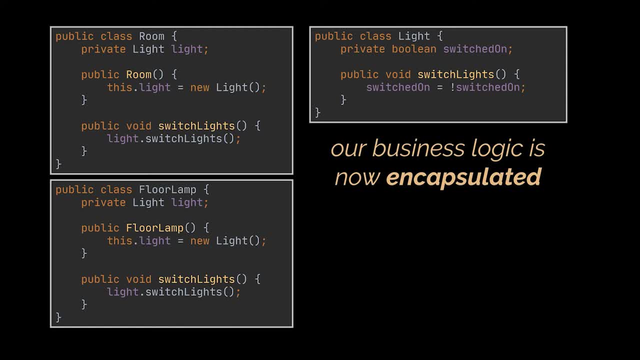 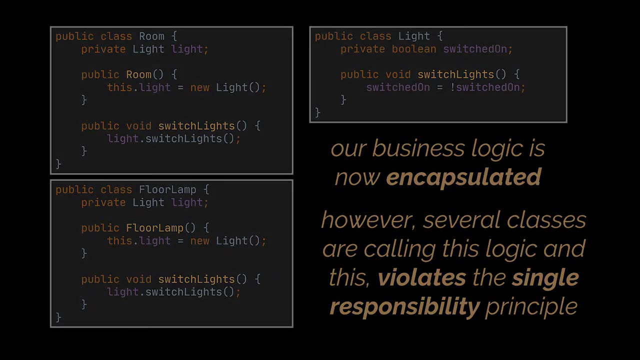 Okay, now our business logic is nicely separated from the rest of our code, but we still have the previous problem. We still have several classes that are calling this logic and switching lights themselves, And this violates the single responsibility principle. To solve this, what you have to do is extract all of the request details from the room class and put them inside the room. 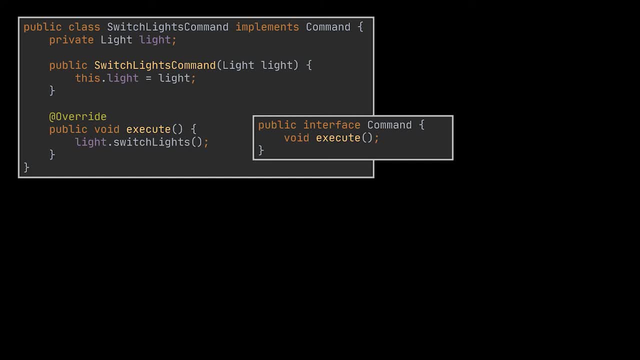 class. You can also put the request details, such as the object being called, the name of the method and the list of arguments passed to this method, into a separate class, with a single method that triggers this request. Classes such as this one host repeated behaviors in our applications and are 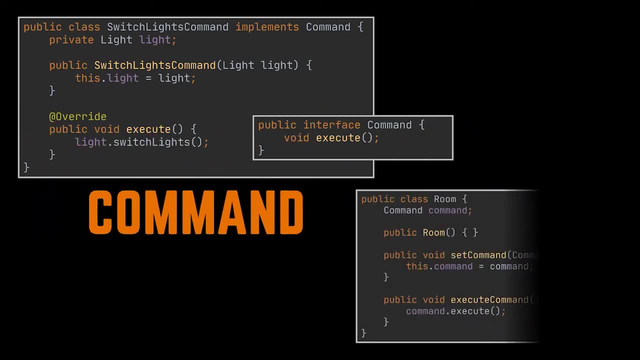 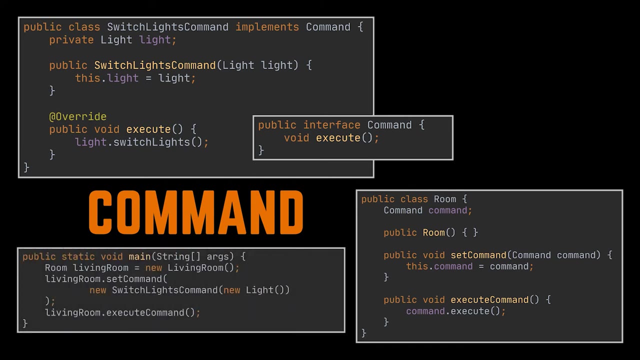 referred to as commands. Now, in this example, our rooms and our floor lamp, as well as any other object we might create, will have a command object as an attribute and an execute command method inside it To switch the light in any of these objects. we set this command to be the switch lights command and execute it. 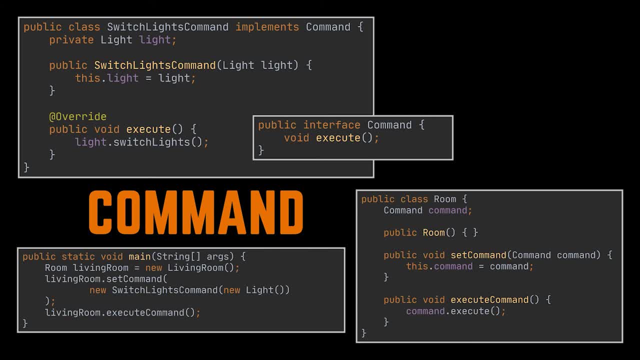 Or maybe later on we can expand on this and pass a list of commands like the close or open curtains command and the open or close door command. The possibilities for extension are endless and on top, of every class has its own responsibility. now, As we manage to decouple the classes that invoke operations from the classes that actually perform these operations, 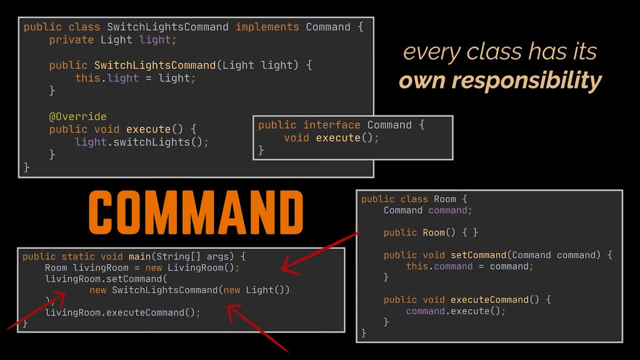 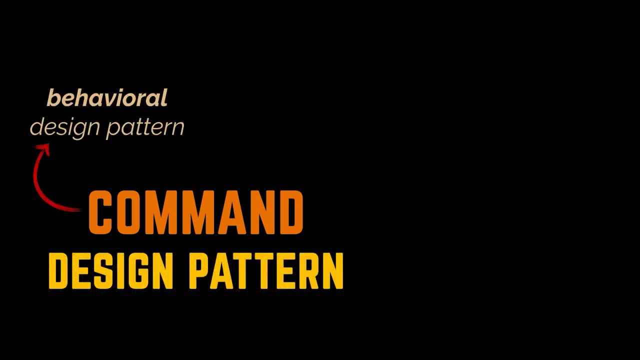 The decisions, assignments and the configuration of our program is now decided at runtime by the client, giving him way more flexibility on how and what to do with the objects at hand, and that's what the command pattern is all about. this pattern is a behavioral design pattern that turns a request. 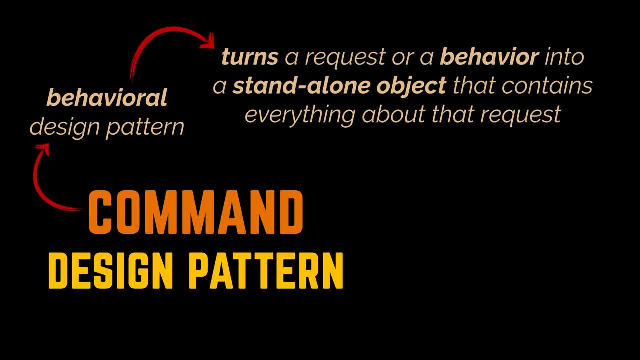 or a behavior into a standalone object that contains everything about that request. it is used to encapsulate all the relevant information needed to perform an action or trigger an event, so that this action may be reused by several parts of our application. okay, let's go ahead now and take a look at the structure, or class diagram of the command design pattern. all while 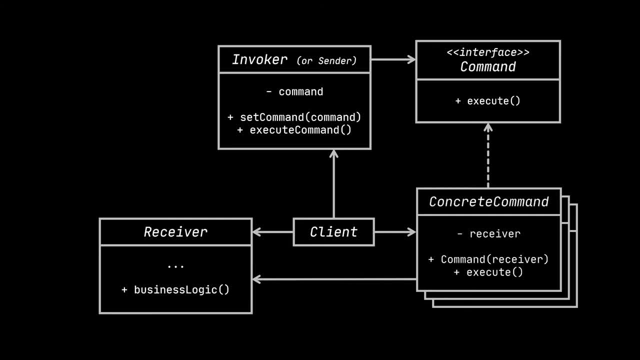 relating it to the house automation example we gave at the beginning of the video. the first thing you will notice here is, of course, the command interface. this interface usually declares a single method for executing the command. next are the concrete commands, which can implement various kinds of requests. these classes can perform the work. 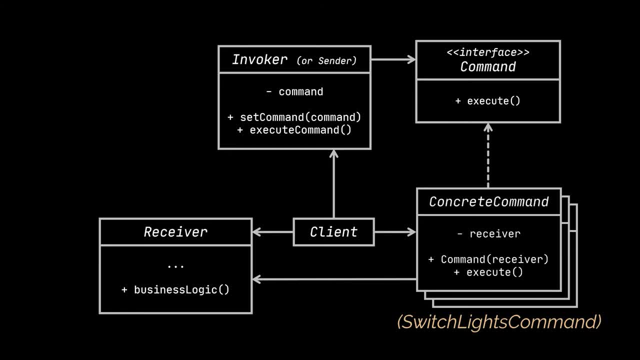 on their own or can pass the call to one of the business logic objects in our application, just like we did in our previous example. now, two terms always associated with the command pattern are the invoker, aka sender, and the receiver. the invoker is responsible for initiating requests. 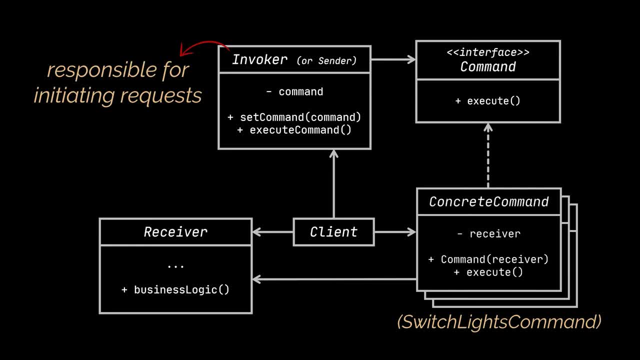 this class must have a field for storing a reference to a command object. the sender triggers that command instead of sending the request directly to the receiver. in our example rooms of the house, where the sender or invoker, however, the receiver class, contains some business logic: almost any object may act as a receiver. most commands only handle the details of how a request 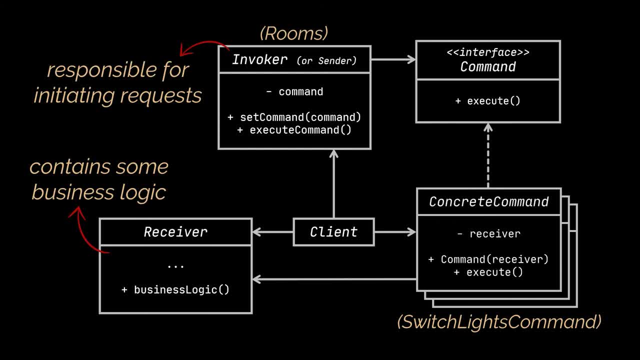 is passed to the receiver, while the receiver itself does the actual work. and that is exactly what was happening in the light class, which was the receiver in our example. the command we created was redirecting the call of the room class to the light class and telling it that it should switch. 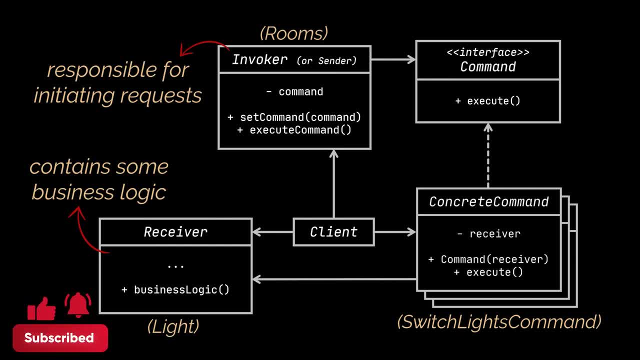 the actual business logic was being done inside the light class and not inside the command itself. finally, the last piece of our class diagram is the client. its responsibility is creating and configuring concrete command objects. the client must pass all of the request parameters, including a receiver instance, into the commands constructor. so to sum everything up, the command.